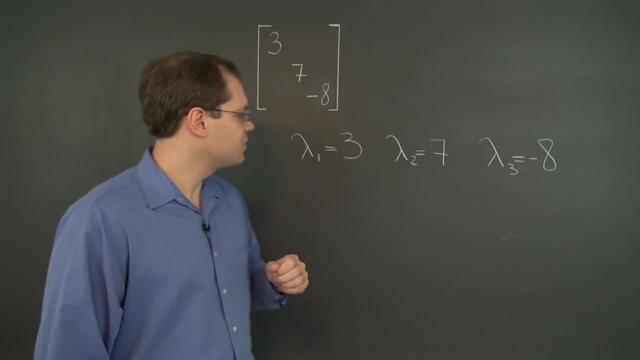 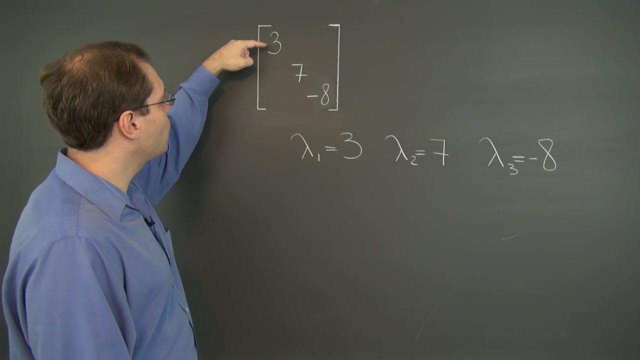 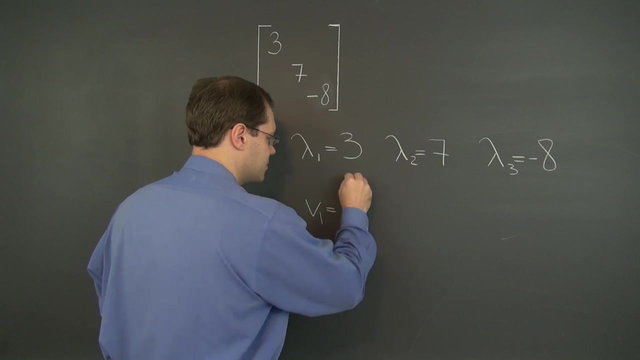 Alright 3,, 7 and negative 8.. And the corresponding eigenvectors are of course for lambda equals. 3, are 1,, 0, 0.. Well, let me write it down and then we'll see why that is v1 equals. 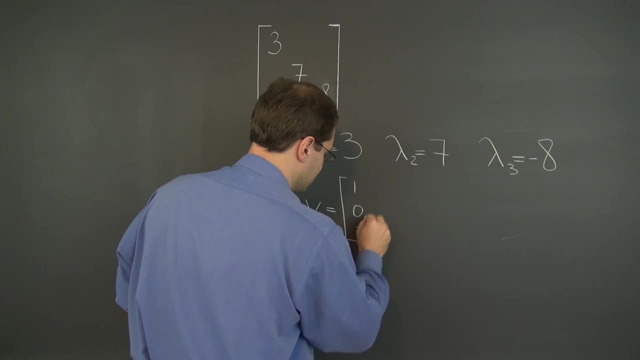 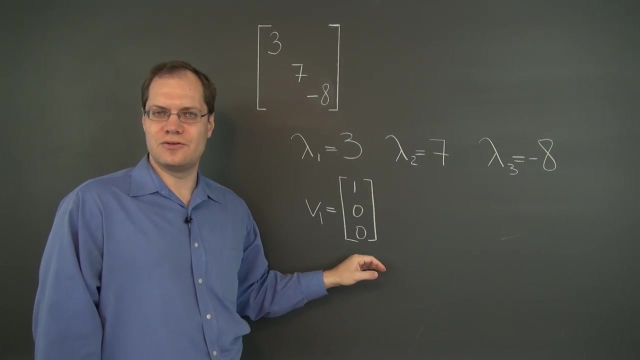 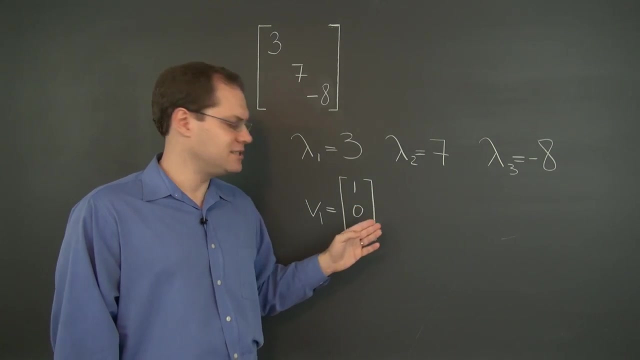 1, 0, 0. And I think it's easy to see why this is the eigenvector, because when you multiply this matrix by 1, 0, 0, the result will be the first column of the matrix and it will be 3, 0, 0, which, of course, is 3 times the input. 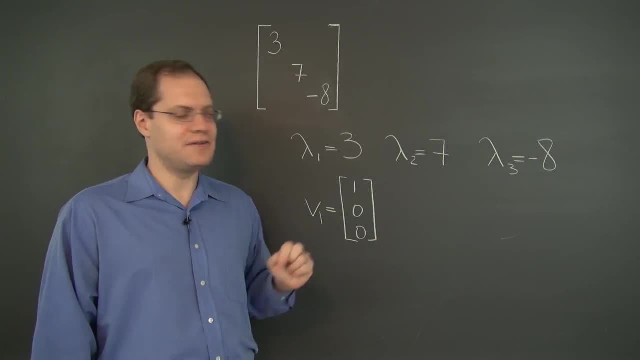 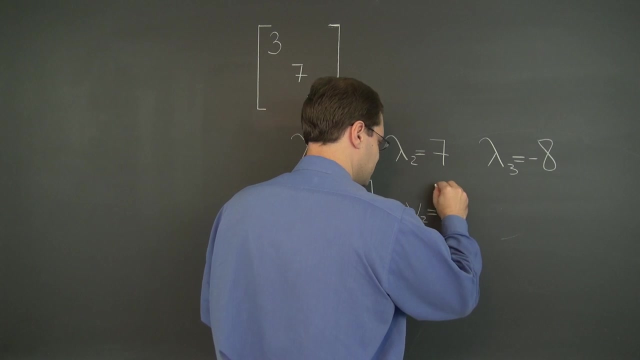 So, indeed, this is the eigenvalue and this is the corresponding eigenvector, And the eigenvector associated with lambda 2 is 0, 1, 0. And the explanation would be just about exactly the same. And finally, v3 would be- you guessed it- 0, 0, 1.. 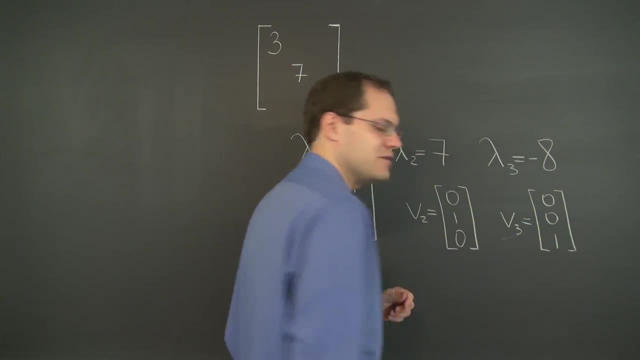 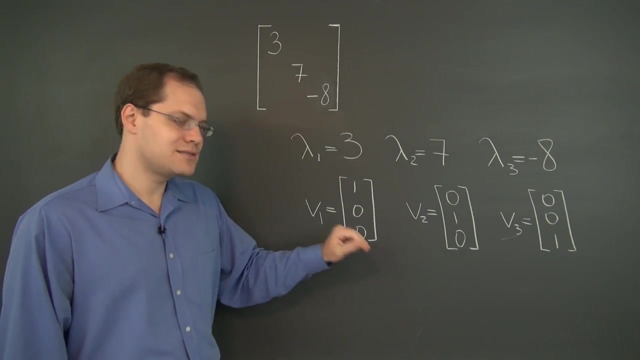 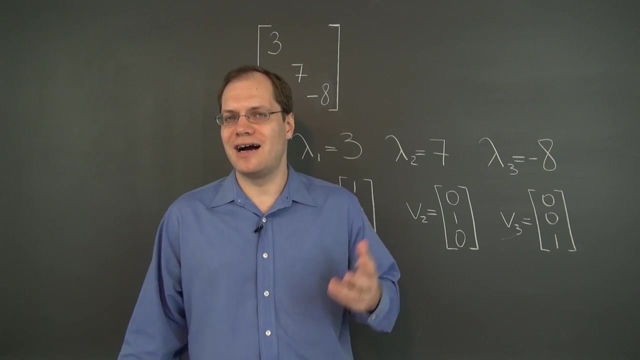 So for diagonal matrices, eigenvalues are right there on the diagonal and eigenvectors are our dream decomposition vectors. You may call this the standard basis for r3 or rn in general. Right, You can also call them our pivot columns, if you so choose, Alright. 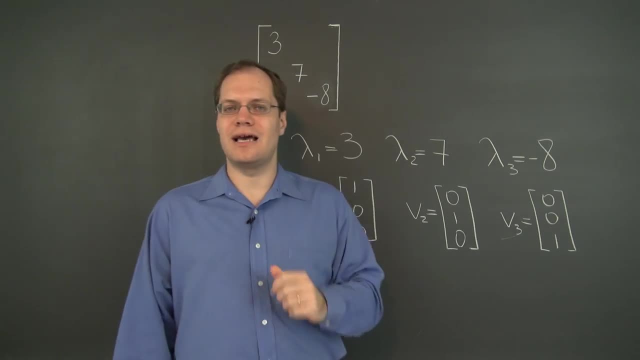 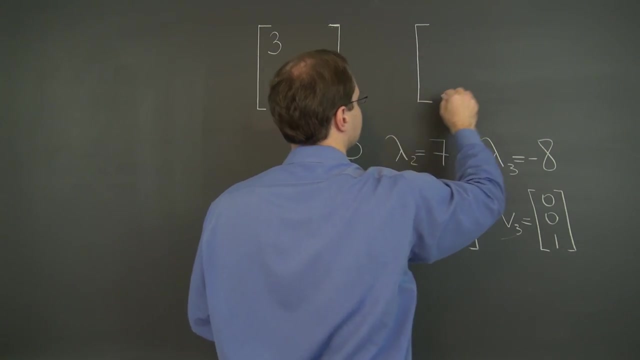 But there you go. These are the eigenvalues and eigenvectors of a diagonal matrix. Now let me ask you an interesting question. Would you say that this diagonal matrix is the eigenvalue? This is the matrix. Same numbers in different order, 7, minus 8,, 3, have the same eigenvalues. 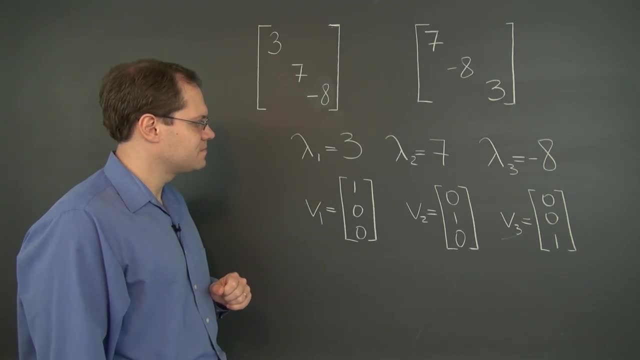 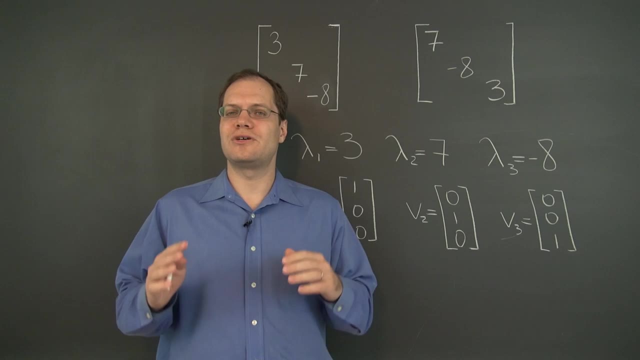 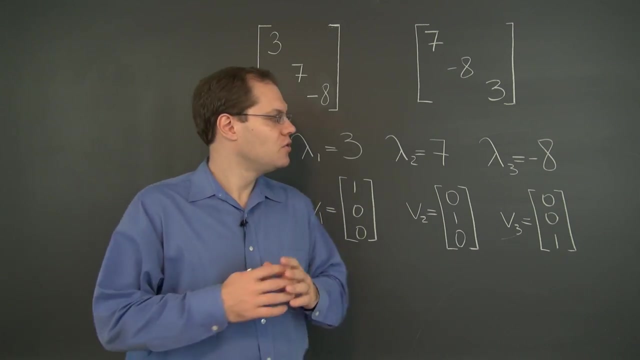 and eigenvectors. Think about it for a moment And I'll bet you, 9 out of 10 said yes, And I'm not going to claim that yes is the wrong answer. I just think that no is a better answer, And here is why. 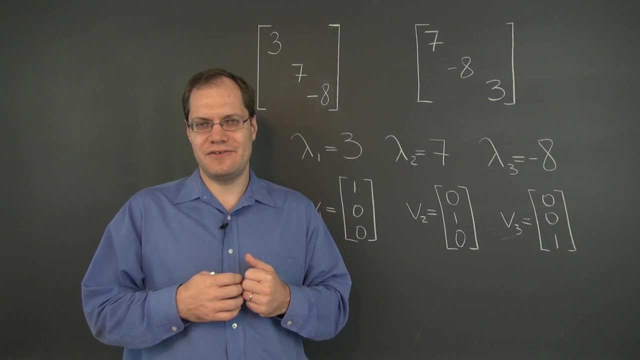 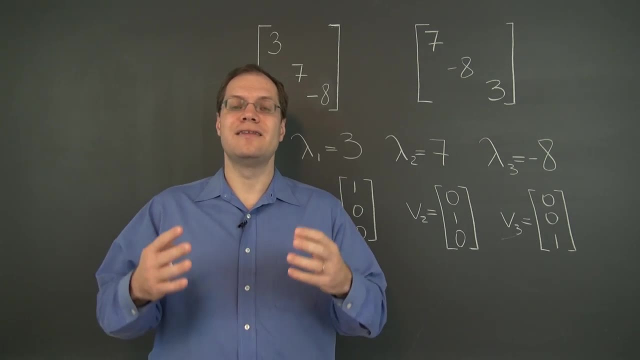 When we say that two matrices have the same eigenvalues and eigenvectors, or if we use the word spectrum, which means the collection of eigenvalues and eigenvectors. When we say that two matrices have the same spectrum, what we mean is not only the fact that the 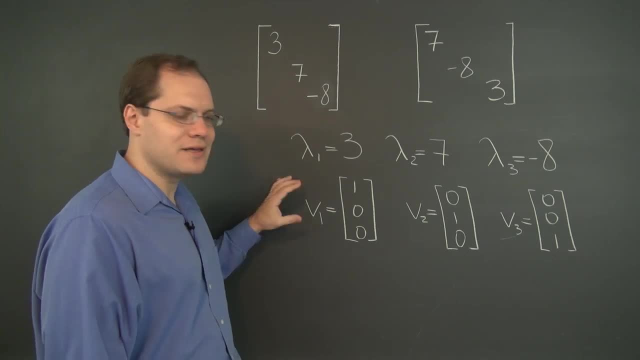 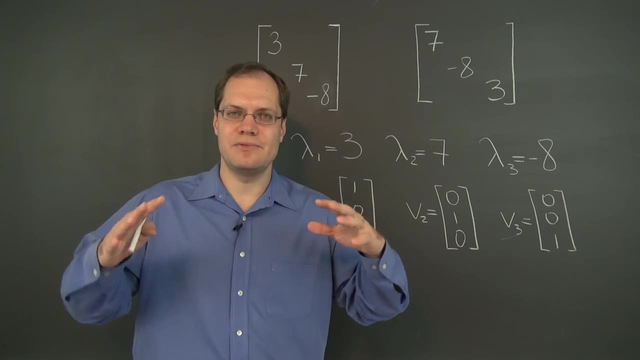 eigenvalues are the same and that the collection of the eigenvectors are the same, but that they are matched up in the same way. also, We want for two matrices to have the same spectrum, we want their eigenvalue eigenvectors to be the same And we want the collection.